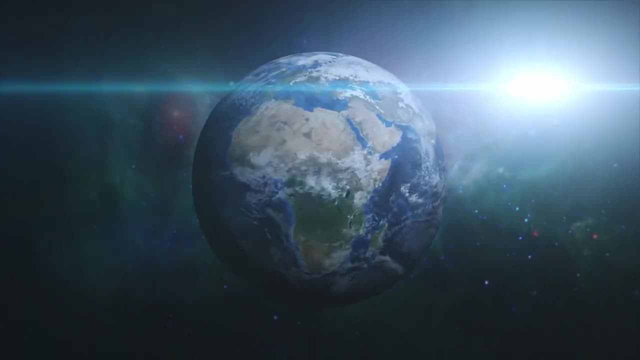 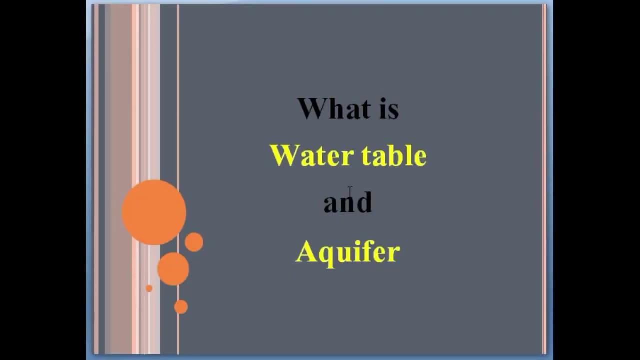 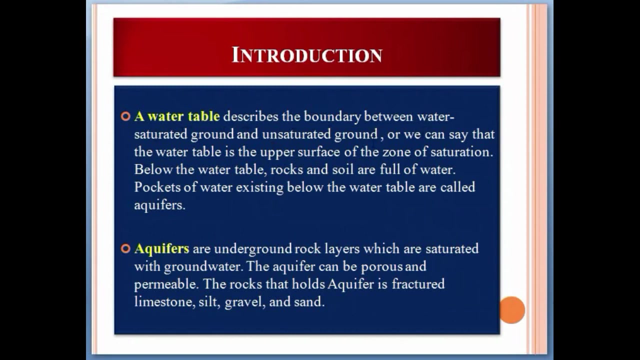 Hello guys. so today we talk about an important topic, that is, water table and aquifers. So in this video we talk about what is water table and what is aquifer. So here is the introduction: Water table describes the boundary between water, saturated ground and unsaturated ground, or we can 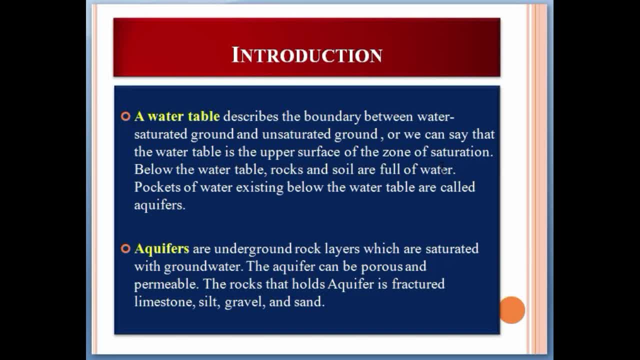 say that the water table is the upper surface of the zone of saturation. Below the water table, rocks and soils are full of water. Pockets of water existing below the water tables are called aquifers. Aquifers are underground rock layers which are saturated with groundwater. The aquifer 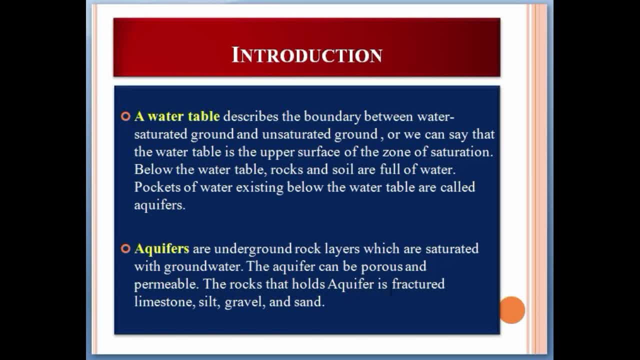 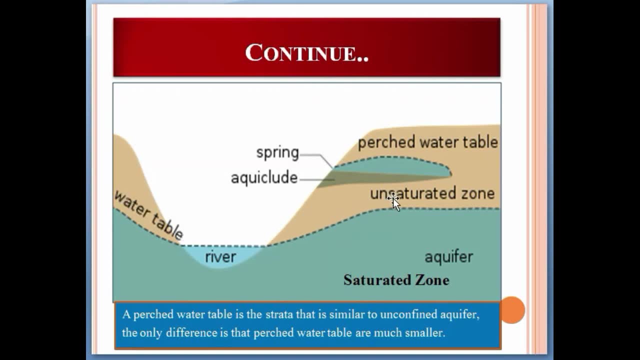 can be porous and permeable. The rocks that holds aquifer is fractured: limestone, silt, gravel and sand. So see here, this is the water table, which is just denoting the boundary between unsaturated zone and saturated zone. So below the water table, the surface is always. 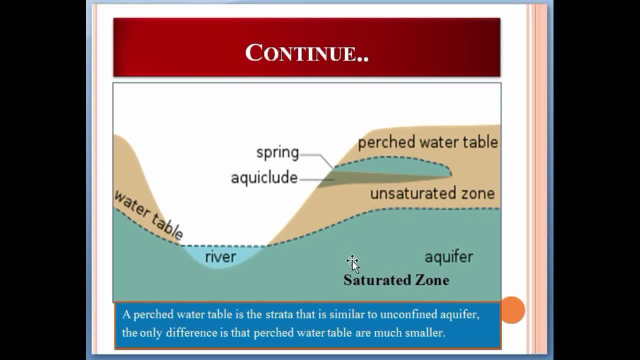 filled with water. As you can see, this is the water and this is the saturated zone Below the water table. some pockets of water is available, which has full of large amount of water. that is known as aquifer. So aquifer is always porous and permeable. The rocks which 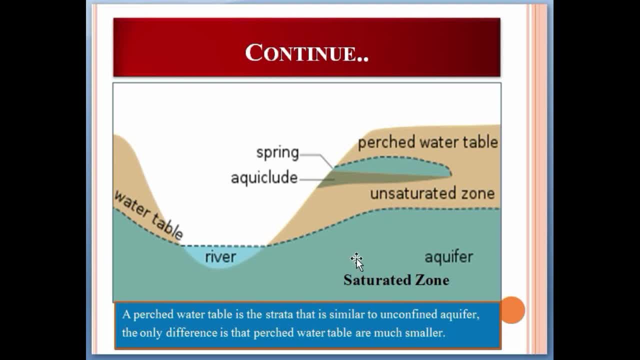 consist actually, aquifer is gravels, sandstone, siltstone or limestone, because sandstone and gravels are always have porosity and permeability. So that's why this zone is actually known as aquifer, A purged water table. So here is the definition of purged water table. I will not 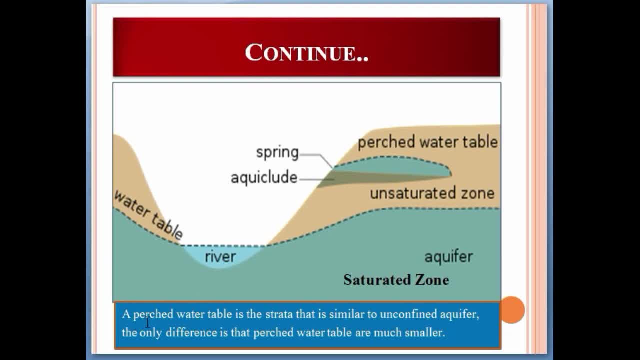 talk much about purged water table in this video. So a purged water table is the strata that is just similar to unconfined aquifer. The only difference is that purged water table are much smaller compared to unconfined aquifer. So actually this is the small portion of 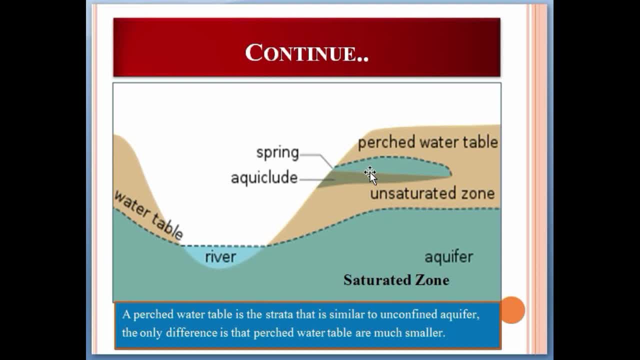 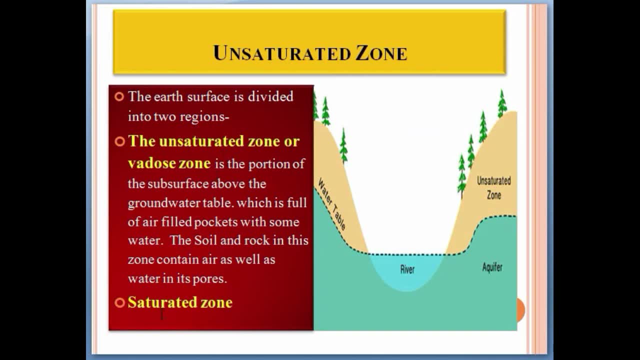 water table that consists some amount of water. The earth's surface is divided into two regions: the zone or wado zone, and the second one is saturated zone. so the unsaturated zone is the portion of the subsurface above the groundwater table which is full of. 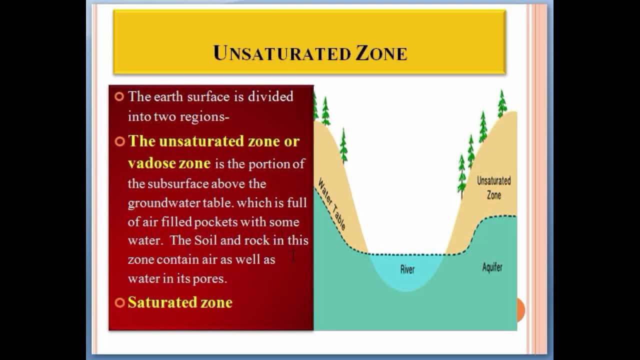 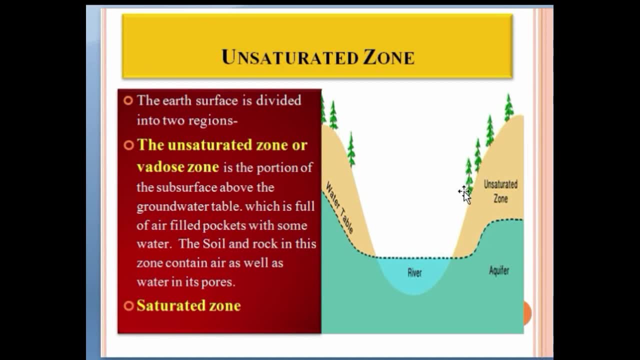 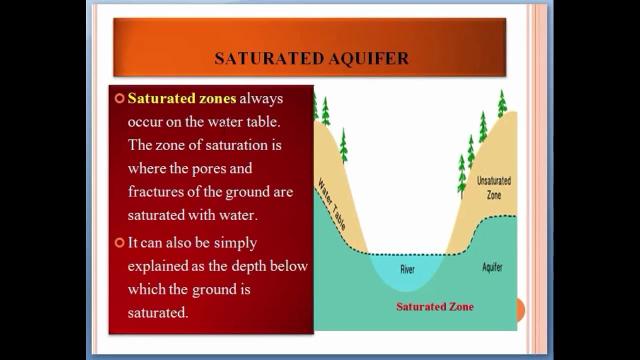 air filled pockets with some water. the soil and rock in this zone contains air as well as water in its pores, so saturated zones always occurs on the water table. the zone of saturation is where the pores and fractures of the grounds are saturated with water. it can also be simply. 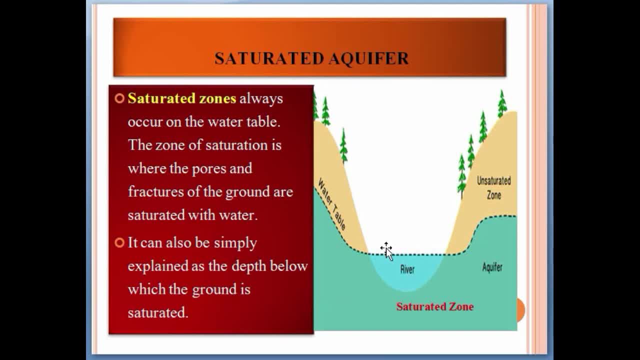 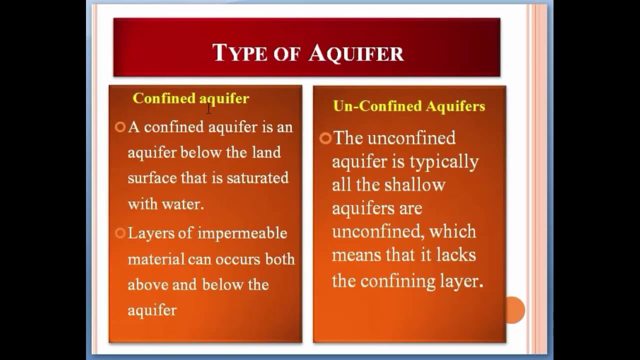 explained as the depth below which the ground is saturated. so this is the saturated zone. so saturated zone always occurs in the water table and this zone is actually consists large amount of water. so this is the difference between unsaturated zone and saturated zone. types of aquifer: confined aquifers and unconfined aquifers. so a confined 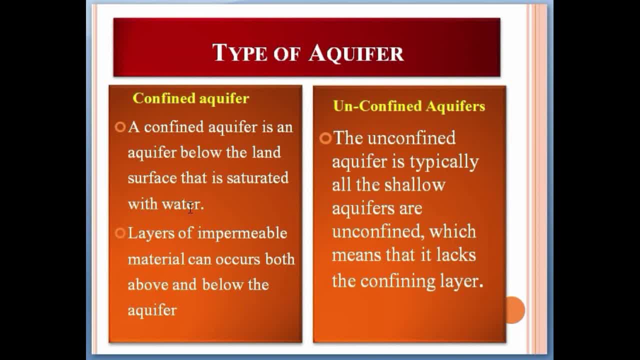 aquifer is an aquifer below the land surface that is saturated with water. layers of impermeable material can occurs both above and below the aquifers. the unconfined aquifer is typically all the shallow aquifers, and that is means that it lacks the 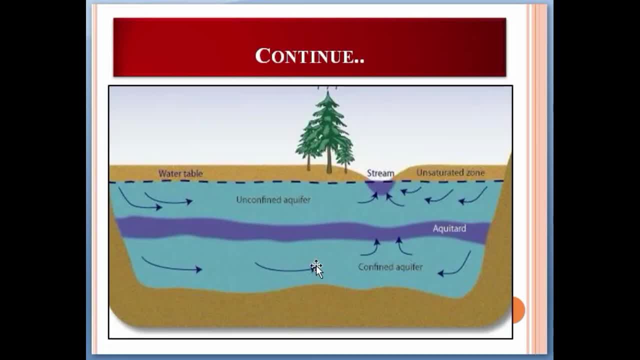 confining layer. actually see here, this is the confining aquifer and this is the unconfined aquifer. so the difference is actually that confined aquifers always have large amount of water, while unconfined aquifer is not a confined aquifer. actually, it means that unconfined aquifers consist some small 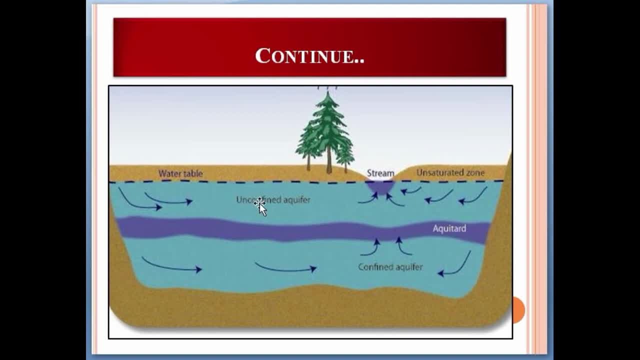 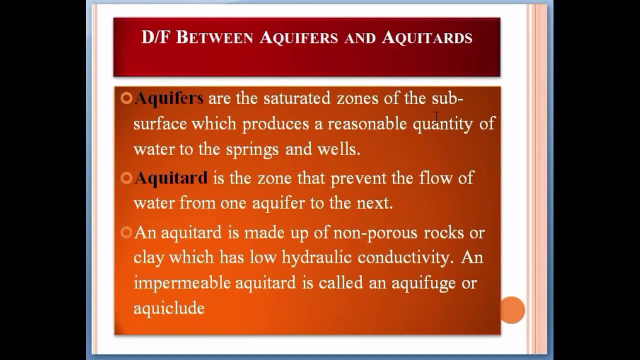 amount of water, or you can say that shallow water table- this is the actually shallow water table- is the first one and the second one is the. while the confined aquifer is actually consist a large amount of water, difference between aquifer and aquitards. so aquifers are the saturated zone of the subsurface which produce 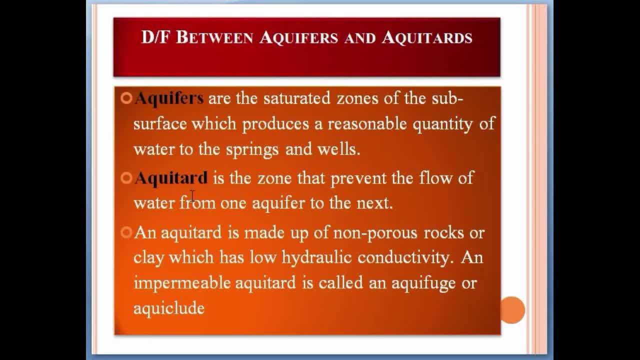 a reasonable quantity of water to the springs and wells, while aquitard is the zone that prevents the flow of water from one aquifer to the next. an aquitard is made up of non-porous rocks or clay, which has low hydraulic conductivity and impermeable equipment is called an aquifuge or.